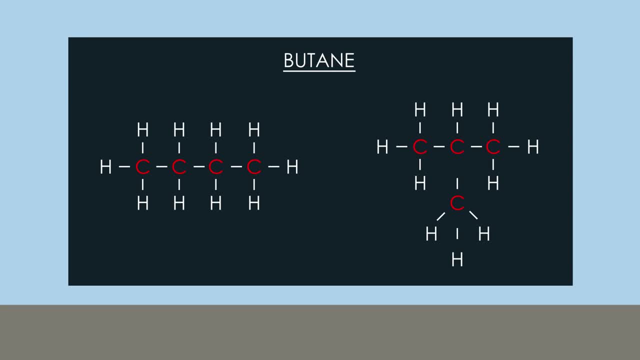 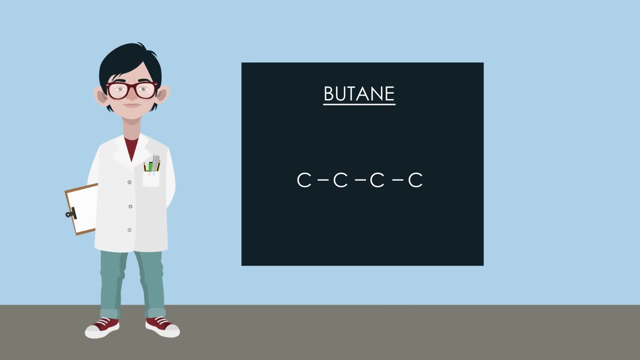 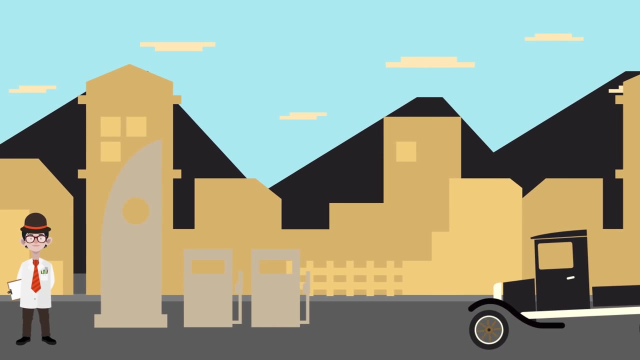 the four carbon atoms. To make it easier to draw these structural formulae, we often omit the hydrogen atoms and just show the bonds connecting the carbon atoms, bending the chain, so you can see where the carbon atoms are Before we try to find more isomers. here is the story of lead-free petrol Petrol. 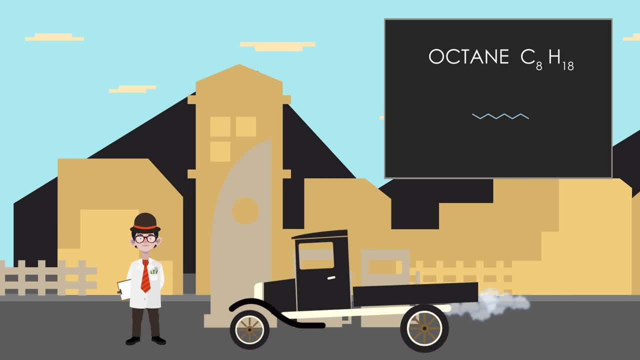 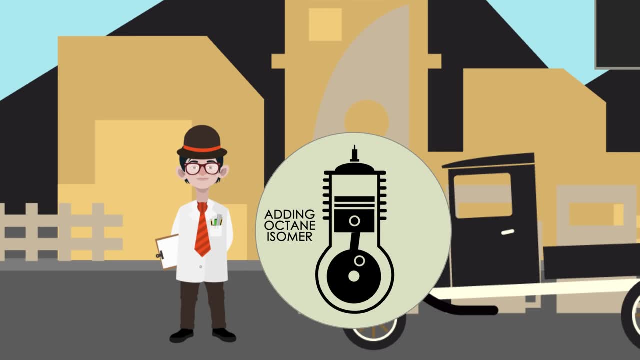 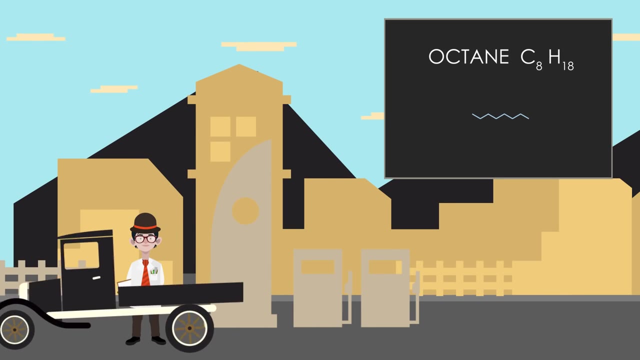 for cars is mostly octane C8H18.. In the 1920s, when petrol started to be used for cars, the petrol-air mix in the cylinders used to explode too quickly before the spark, causing the engine to knock or jolt If an isomer of octane was used. the 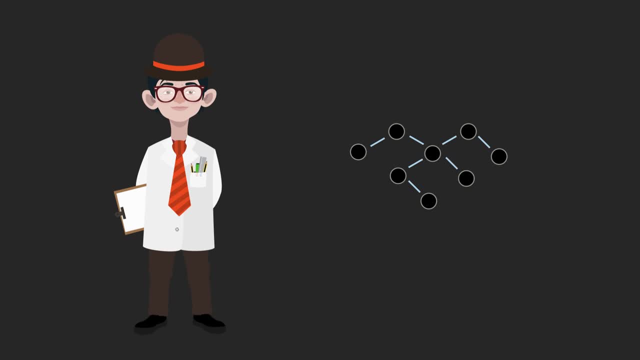 petrol burnt more smoothly. Look carefully, there are eight carbon atoms, so it is a structural isomer of octane. but what is its formal name? Pause and count the atoms in the longest chain. Whichever way you count, the longest chain is five carbon atoms long, so the name will be pentane, And off the third atom in the. 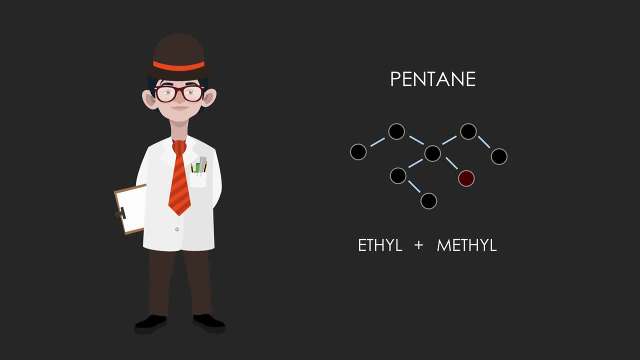 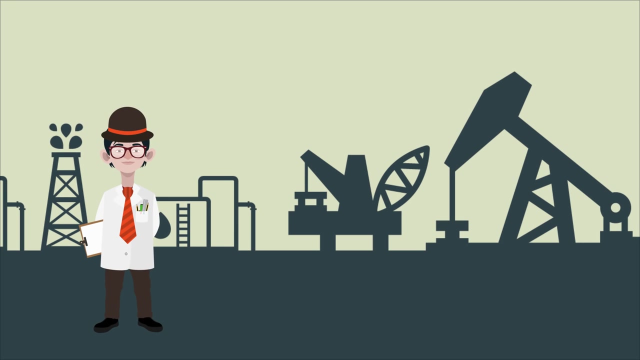 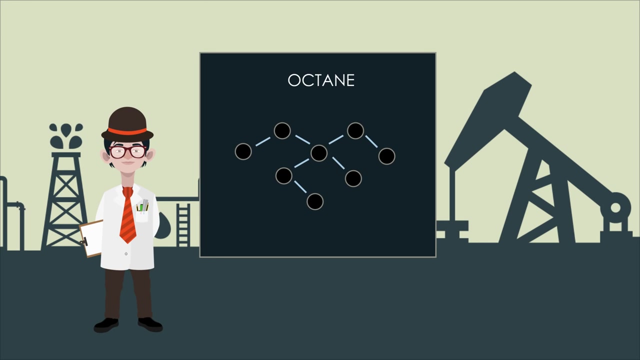 INA chain. there is an ethyl group and also a methyl group, so its name will be three, three methyl ethyl pentane, But this compound is not normally found in crude oil and is very expensive. In 1923, scientists discovered a compound of lead with almost the same structure and did the job perfectly. 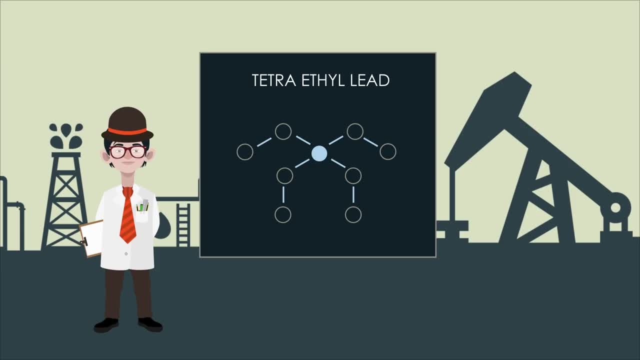 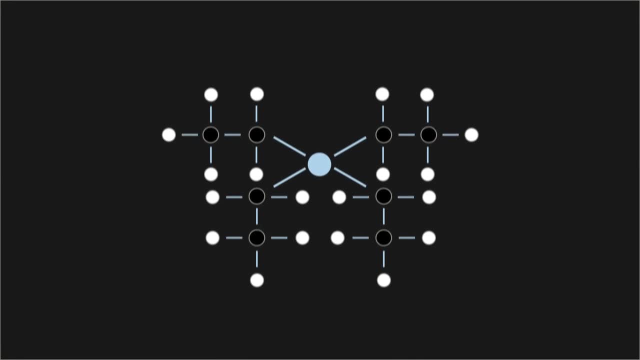 LED-tetraethyl laws or tetraethyl lead. You might remember that lead is in group 4 of the periodic table along with carbon. The lead addition helped the petrol to burn smoothly, but the lead atoms combine with oxygen, forming lead oxide. This comes out. 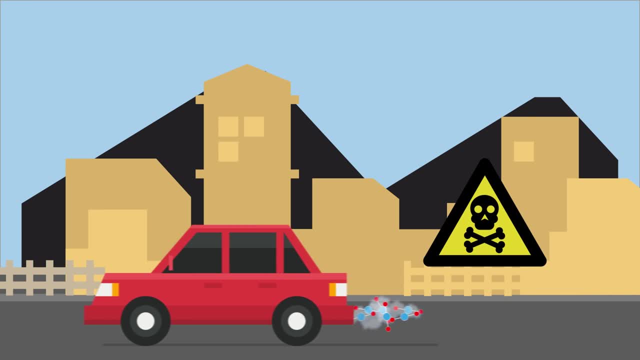 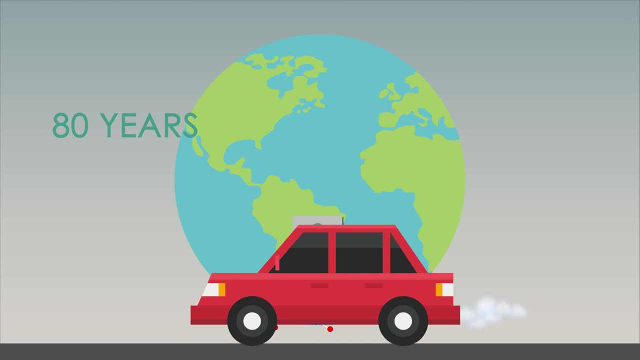 of the exhaust pipe as a fine dust and is very toxic. It has taken us until this 21st century to get rid of all the lead in petrol globally, But for 80 years lead from car exhausts has been carried around the world and is even found in. 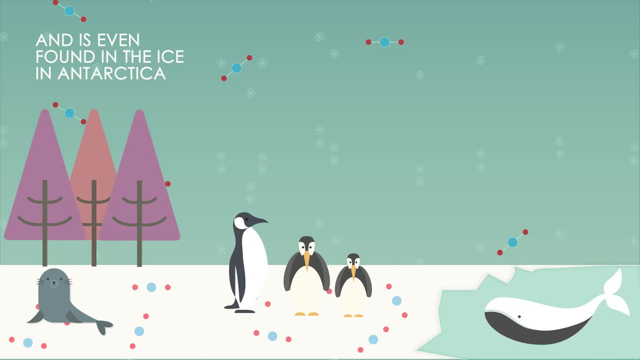 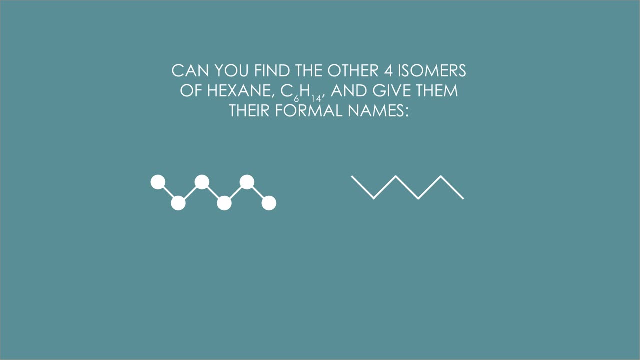 the ice in Antarctica. So let's finish with a simpler example. Can you find the other four isomers of hexane, C6H14, and give them their formal names? I'll give you a hint. There are two based on pentane and two based on butane. Pause.